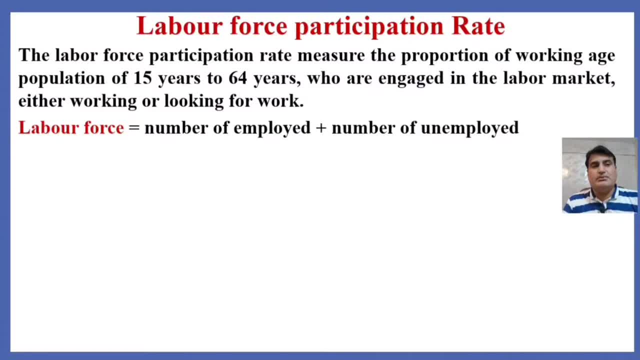 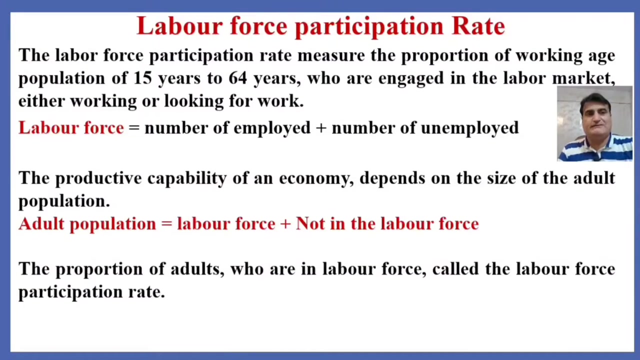 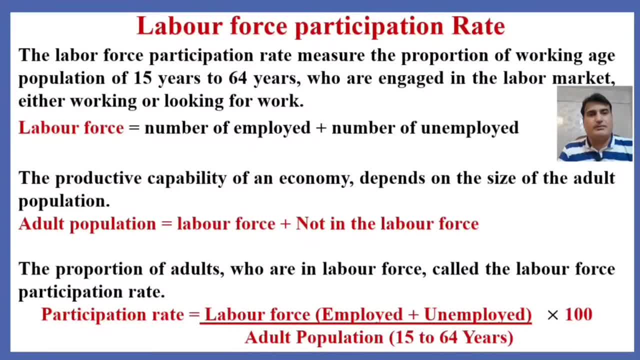 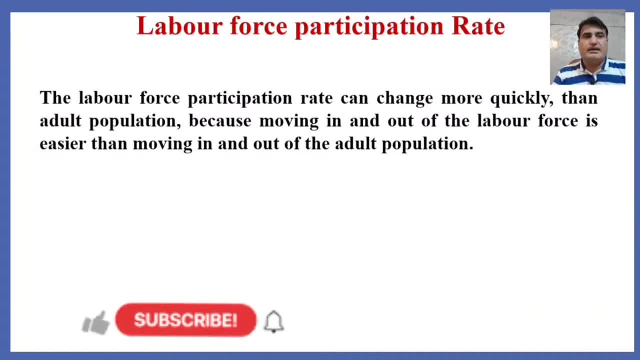 The labor force participation rate formula is the ratio of the labor force to adult population multiplied by 100. The labor force participation rate can change more quickly than adult population. Moving in and out of the labor force is easier than moving in and out of the adult population. 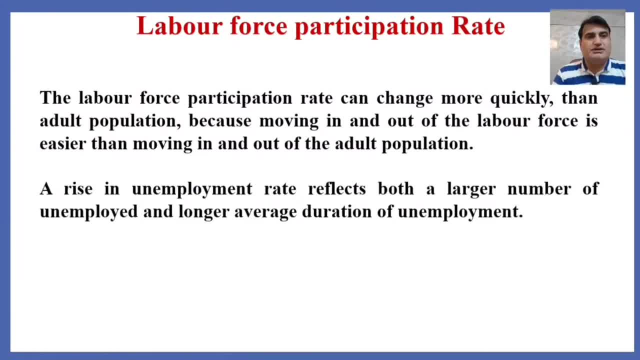 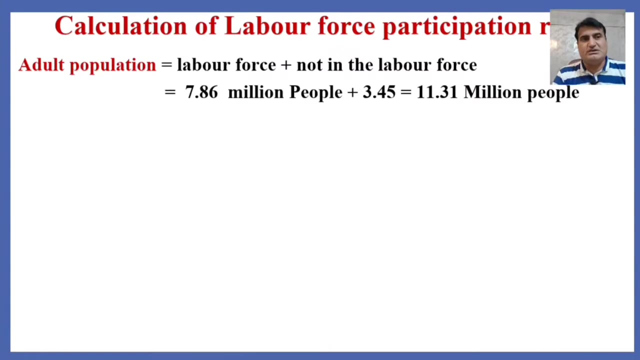 A rise in unemployment rate reflects both larger number of unemployed and longer average duration of unemployment. The labor force participation rate shows the supply of labor available for production of goods and services. How to calculate the labor force participation rate as we calculated the adult population in underestimation and overestimation of unemployment. 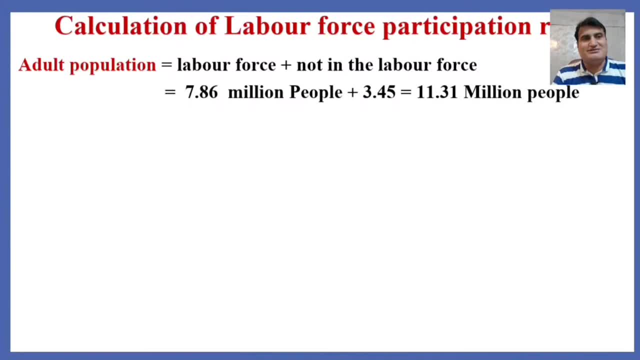 If you want to test your knowledge about underestimation and overestimation of unemployment, you can use the labor force participation rate formula. You can watch my video on underestimation and overestimation or limitations of unemployment rate. The link is given in the description box. 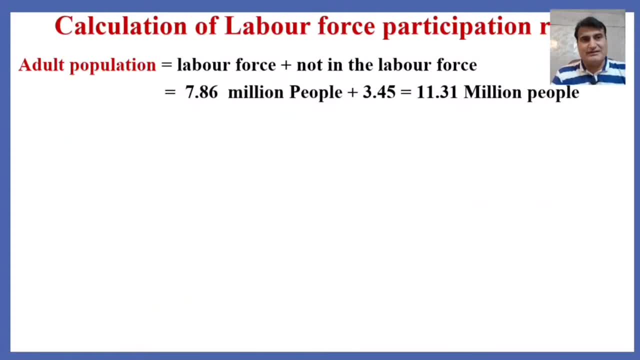 Adult population is equal to labor force plus not included in labor force: 7.86 million are the labor force who are employed, plus unemployed people. 3.45 million people are those people who are not working due to any reason, whether they are full time or not. 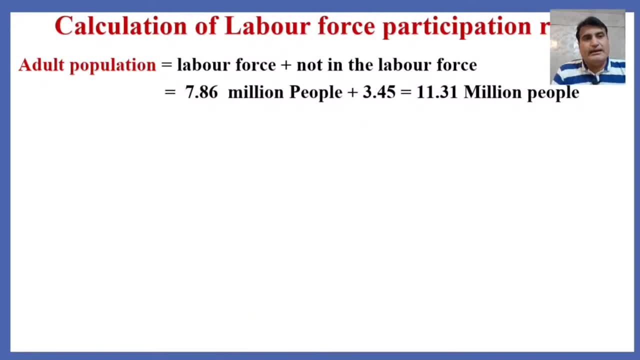 So the labor force participation rate is equal to labor force participation rate In the case of those who are full time. students are suffering from illness and lying on bed rest for longer period. The total adult population is 11.31 million people. The labor force participation rate is the ratio of the labor force to adult population multiplied by 100.